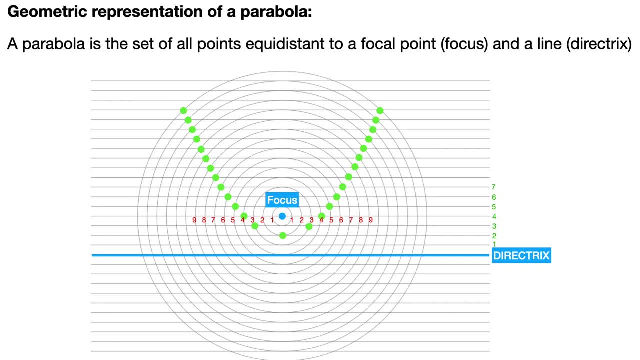 circle and fifth line and so on. All these points are equidistant from the focus and the directrix and a parabola is formed. So you can see that, in fact, a parabola is the set of all points equidistant from a focus. 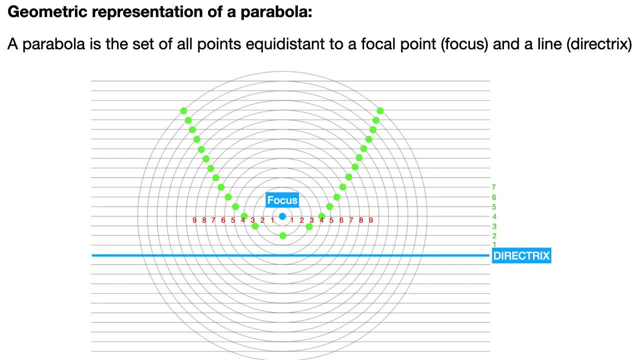 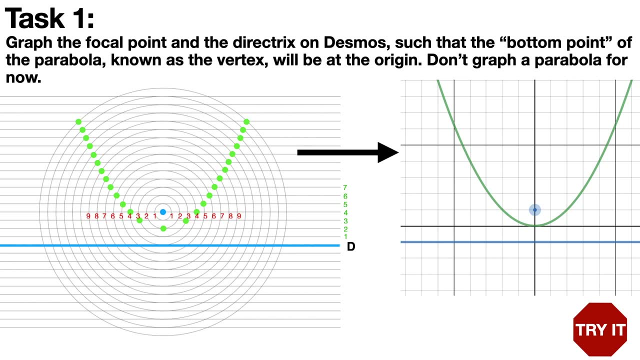 So you can see that, in fact, the parabola is the set of all points equidistant from a focus and a directrix, focal point and a line. The purpose of today's lesson is to be able to translate this geometric definition of a parabola into algebra, And we'll be doing this in a series of tasks. 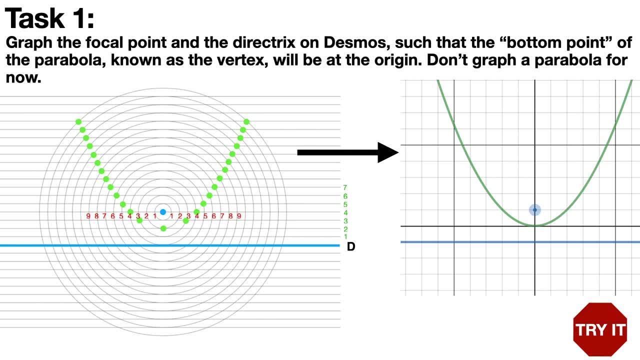 And so the first thing I'm going to ask you to try to do is to graph on Desmos the focal point and the directrix And try to have it so that the center, so to speak, the vertex of the parabola will be at the origin. But don't actually graph a parabola for now. 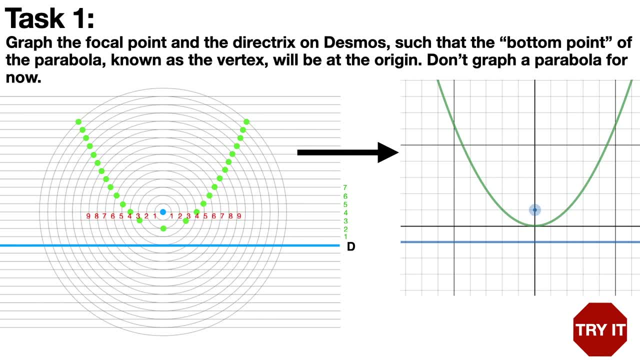 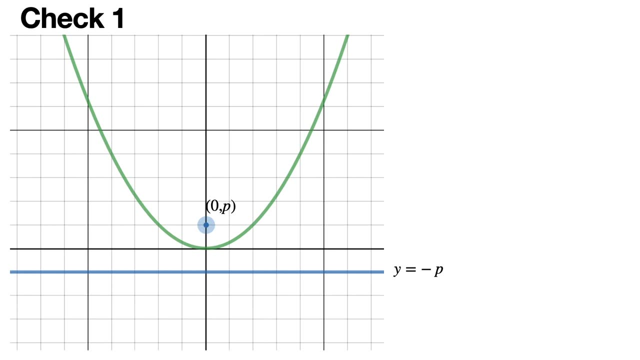 Just see if you can graph the focal point and the directrix. Did you try it? Let's see what you could have done. So, first off, we never really said how far the focus is from the origin and how far the directrix is from the origin. 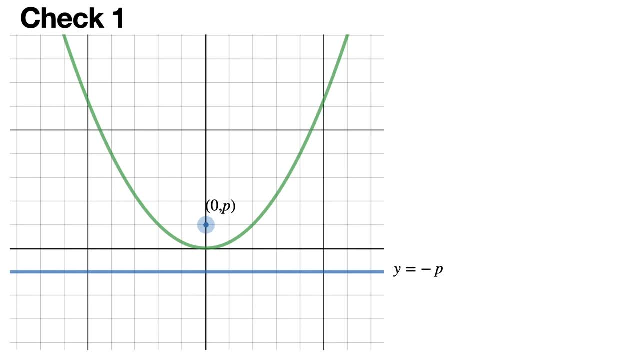 So in these cases, we would want to give a focal point and a directrix. And we would want to give a focal point and a directrix To assign it a variable, in this case p, a parameter, And that distance can change as you. 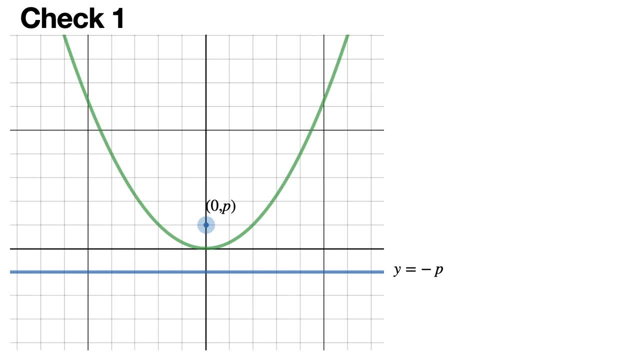 adjust p on Desmos And if you have p be positive, then in order for the line to appear below, that would have to be y equals negative p. So you'd have to know a little bit, remember how to get a horizontal line, in order to do this task properly. 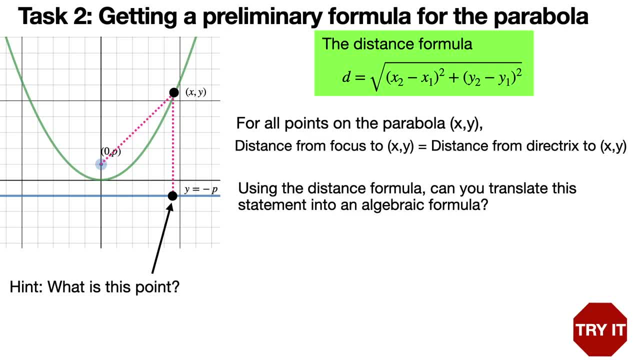 So the second thing I'm going to ask you to do is to give a focal point and a directrix. The second thing we're going to do is we're going to get a preliminary formula for the parabola that has that focus and that directrix, And we're going to use the definition of a parabola to do. 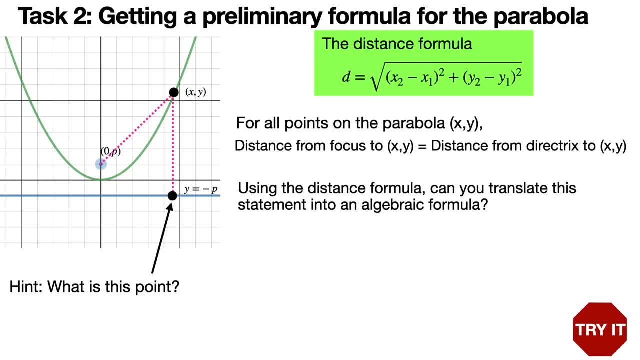 this. So a definition of a parabola is all the points, such that the distance from the focus to the point is equal to the distance from the directrix to the point, And using the distance formula, can you translate this statement into an algebra? 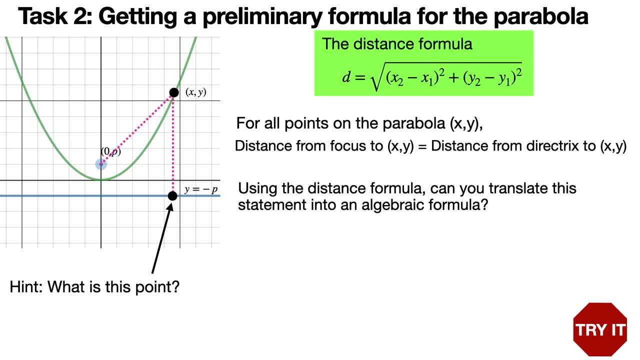 So the distance formula is above there. If you don't remember how the distance formula works, you can check out one of the appendices at the end of this video for a refresher on the distance formula. So try to use the distance formula to translate that sentence: distance from focus to. 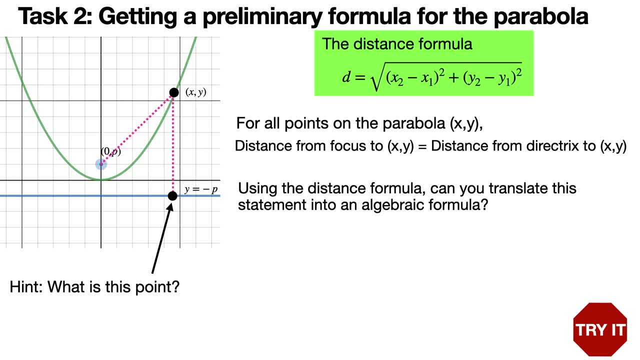 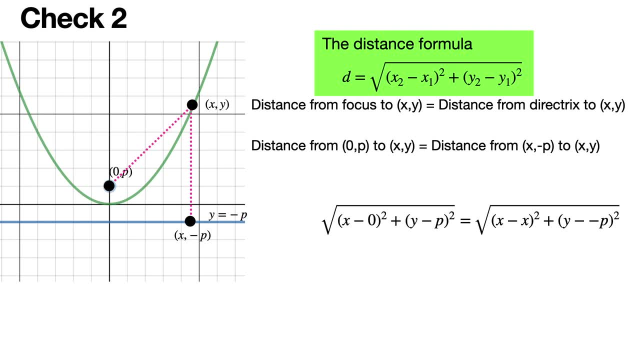 xy is equal to distance from directrix to xy into an algebraic equation. Try it. So if you carefully use the distance formula and you plug in your points, then that's really all there is to this. The other part is that the point on the directrix is x negative p, So the x value is x. 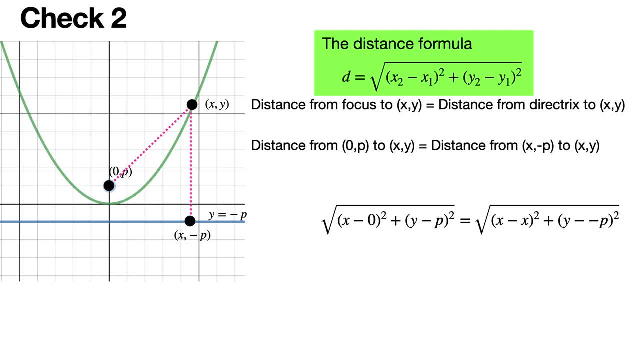 and because it's on the line, y equals negative p. the y value is negative p, So that point on the line is x negative p. So you very carefully plug in your points and it doesn't matter which point you use first or which point you use second. 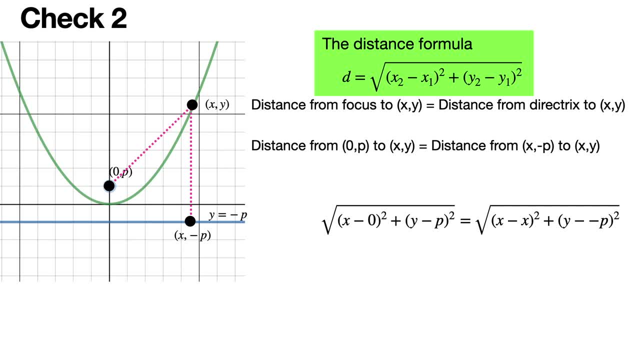 because when you square it you get x. So you plug in your points and you plug in your points and you square it. all the differences are going to be made positive, no matter what. So if you're careful enough, you'll have some sort of version of this Now, depending on order. 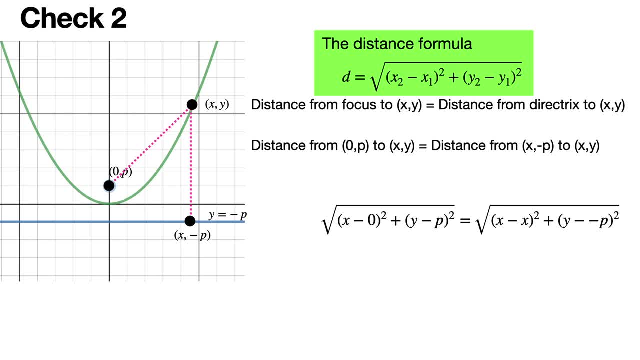 yours might look a little bit different, but it shouldn't matter in the end, And the only thing that might make a difference is the order in which you put some of these things. So you'll see whether you're right if you try the next task. So, believe it or not, this formula. 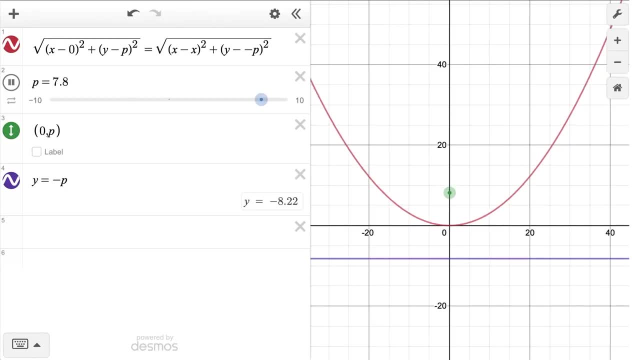 as kind of unattractive as it is, is actually enough for, on Desmos, the parabola to be formed. This is not a nice version of the formula. It is unsimplified and rather inelegant, but this is a formula for a parabola, And so our last task is going to be to make this into a slightly more. 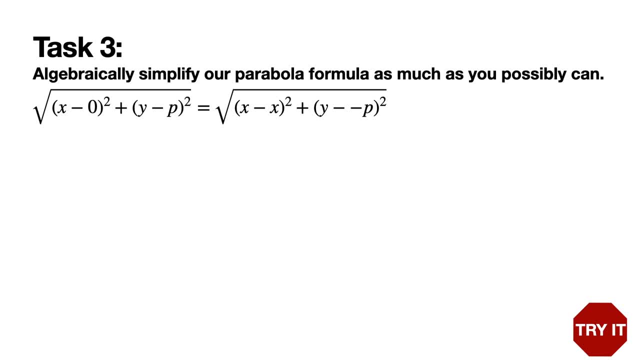 elegant formula. So task number three: take this formula for a parabola with a vertex at 0,, 0, and distance from the focus to the vertex p, and simplify it as much as you possibly can. So try it. You might not get all the way with it, but it's really important for you to try it. 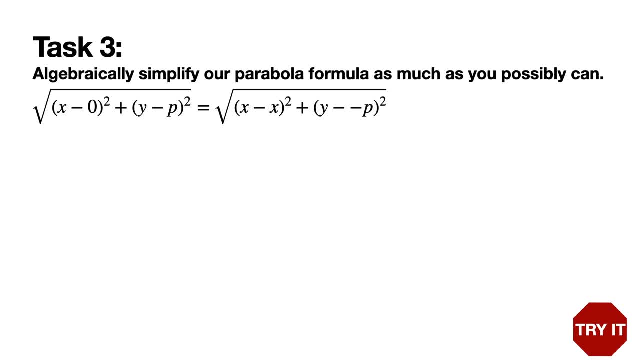 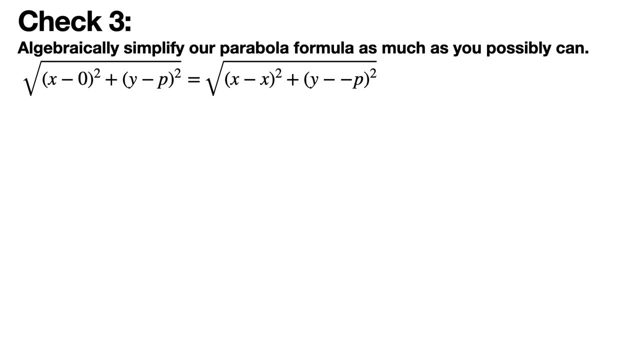 yourself. first, Can you simplify this thing? So we are going to go over the algebraic steps of how to simplify this. First, you can square both sides. Both sides are square roots. Squaring is the opposite of taking a square root. So you can simply eliminate the radicals entirely. 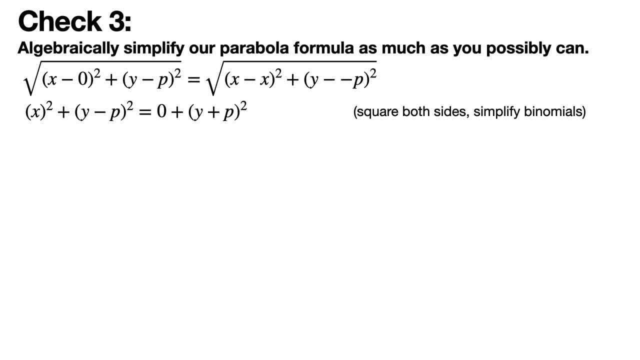 And the other change that I made was I made the y minus negative p into y plus p. Some of you probably did that already. That's fine. So now, what should we do next? And unfortunately, we need to be able to expand binomials and not be. 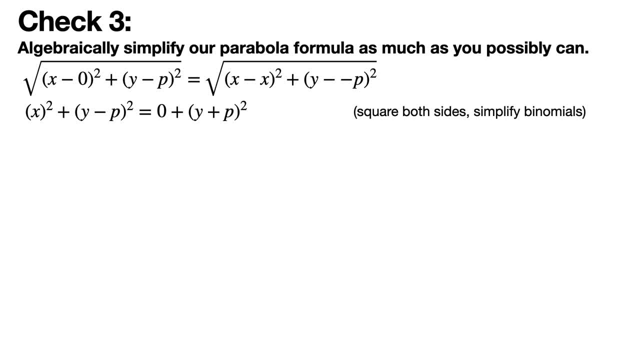 scared of it. So if you got to this stage and then stopped because you were afraid of going forward, you got to push on ahead. You expand the binomials. If you do not know how to expand a binomial or multiply an expression by another expression, then see one of the appendices at the 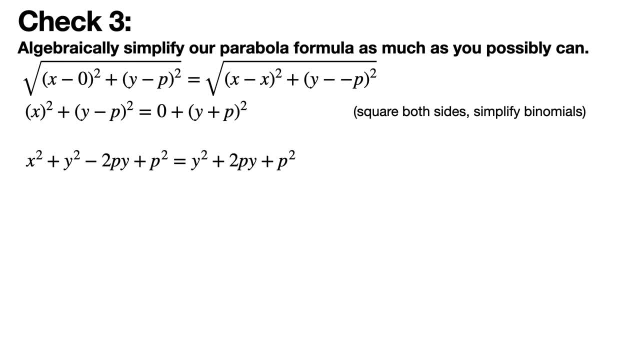 end, Appendix number two. So what to do next? You have this longer thing. You can notice that there are the same things on both sides being added. So you can subtract those things from both sides, which is a legal algebraic move. You get x squared minus 2py is equal to 2py. 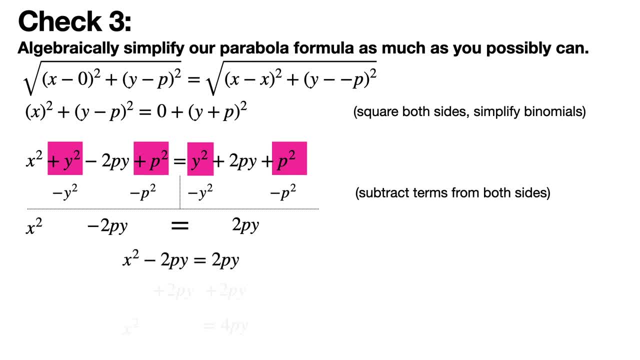 And then x squared minus 2py equals 2py. You can simplify this a little more, if you want, by adding 2py to both sides to get a rather nice formula. x squared is equal to 4py. So this is the. 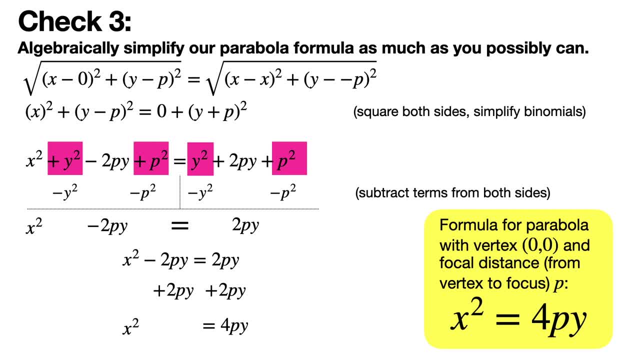 formula for a parabola with vertex of 0,, 0 and the focal distance from vertex to focus or from vertex to directrix, p is x, squared is equal to 4py. Notice that in this formula there's no y. 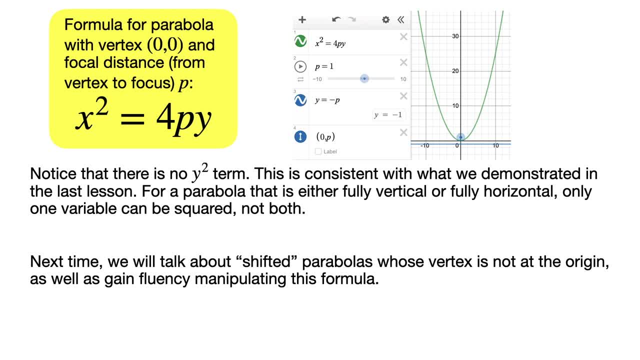 squared term, There's only an x squared- And this is consistent with what we demonstrated in the last lesson- For a parabola that is either fully vertical or fully horizontal. in other words, it's not like those rotated parabolas that we 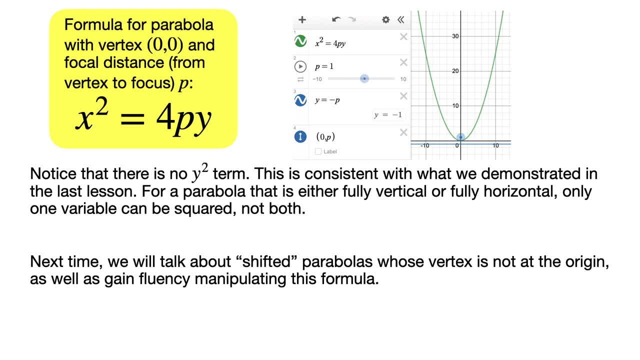 briefly saw in the last lesson, Only one of the variables can be squared, but not both. And in fact, if you want to have a horizontal parabola, it's the y squared is going to be the squared term and x is going to be the one without a square. Next time we're going to talk about 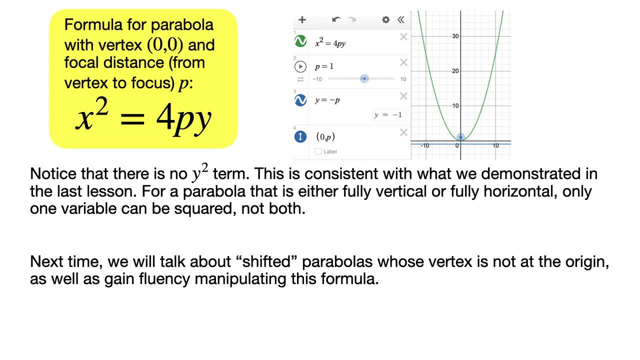 shifted parabolas whose vertex is not at the origin, as well as gain fluency manipulating this formula. Until then, have a great day. And if you were confused about some earlier skill required in the lesson, you can click on the link in the description below to learn more about. 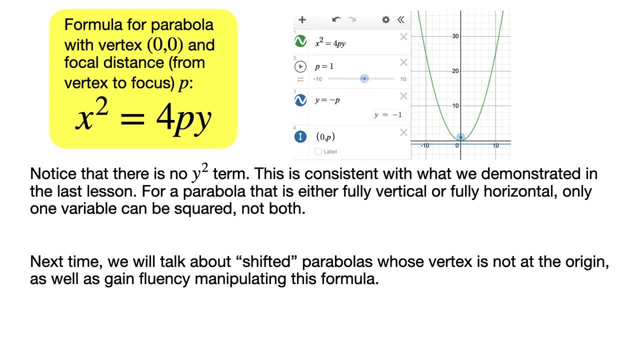 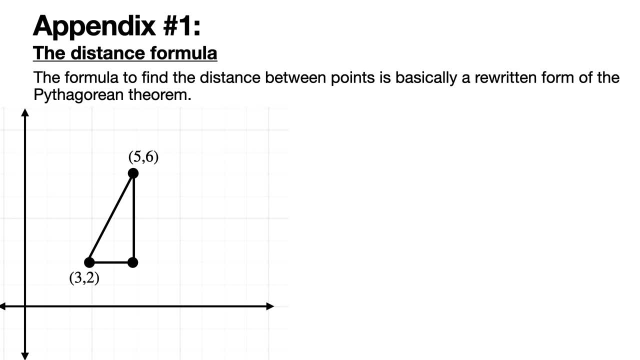 these new products available for-use and further learning about this new stock. Appendix Number 1. The Distance formula. So if you want to find the distance between two points in 2D space, the formula to find the distance is basically the Pythagorean Theorem. 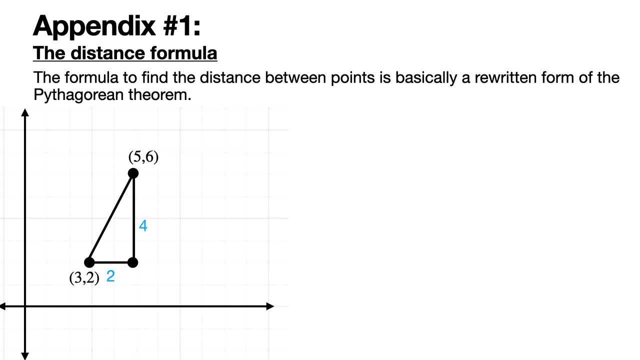 We're going to do this twice, so you get the idea. The Pythagorean Theorem is: a squared plus b squared is equal to c squared and the distances are clearly two and four. so you just plug them into the formula And you can take the square root of both sides at the beginning, an bigger from the. 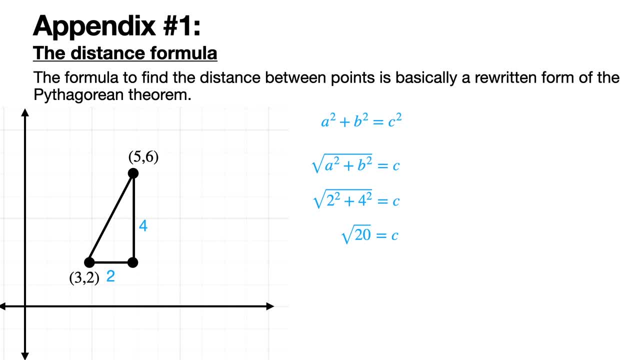 to make it slightly easier and you get: the square root of 20 is going to be c. So this is pretty elementary if you know the Pythagorean theorem, and if you don't know that, then you should watch videos on the Pythagorean theorem until you have the idea. But what if, instead of 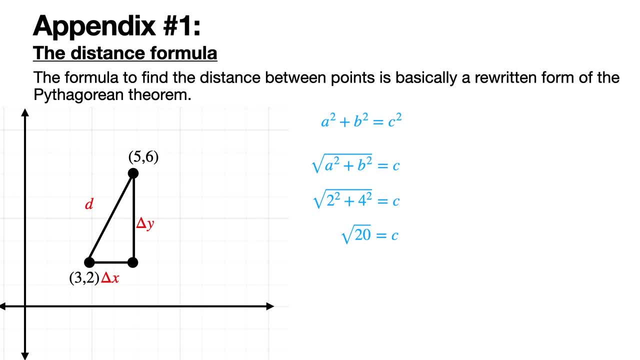 calling it by a, b, c or by 2,, 4,, and whatever the answer is square root of 20,. we called it delta x, delta, y and d. So delta x, delta in math means change, and so the change in x is literally. 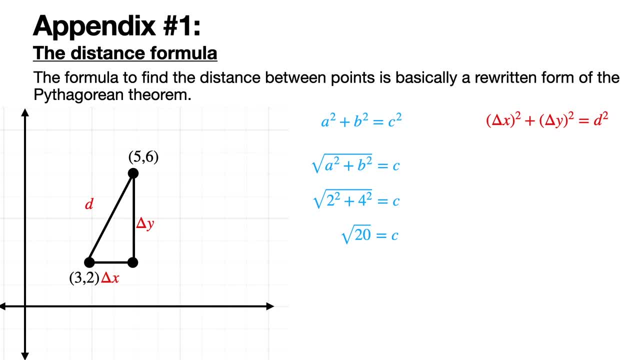 the distance between in the bottom side of that triangle and delta y is the distance of the tall leg, the vertical side of the triangle, and it's equal to d squared. So all we did was we changed the Pythagorean theorem and gave it new names, and if we took the square root of both sides, 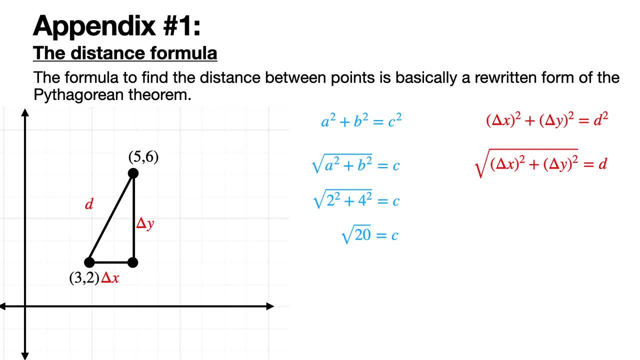 we would get what is essentially the distance formula. Now this delta x. the only thing that's left is to say: how do we find the distance between the x values of those two points? How do we find delta x and delta y? 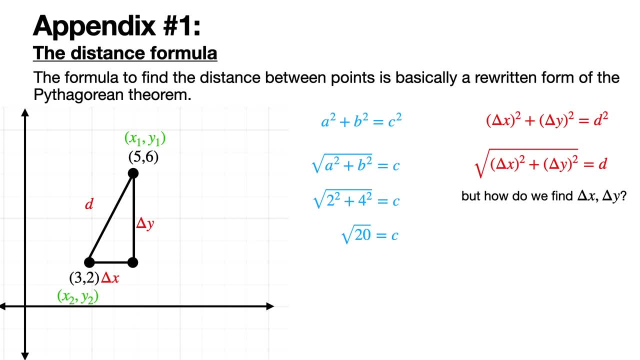 And the answer is we use the two points we're given in green: x1, y1, x2, y2, whatever they happen to be, and delta x is the difference of the two x values and delta y is the distance of the. 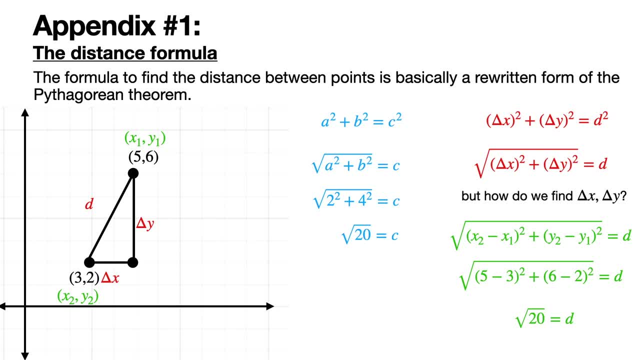 two y values. So all we need to do is carefully plug in the points into the formula and we won't even know the difference between the two x values. So we're going to use the formula and we're going to need to draw a triangle and visually see how long the sides are. We can just do the 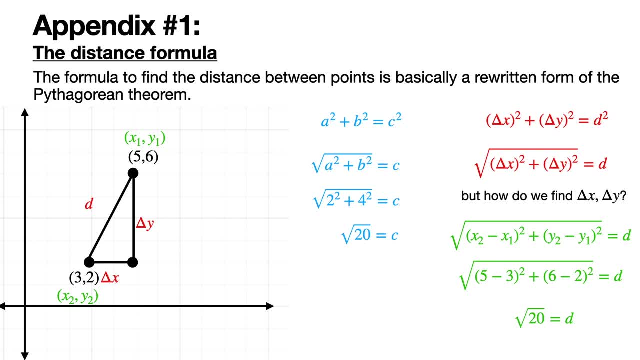 math. So 5 minus 3 is 2, and 6 minus 2 is 4,, just like in the first one, and you can, just if you have the points, not draw a picture and get the answer algebraically. So that's what the distance. 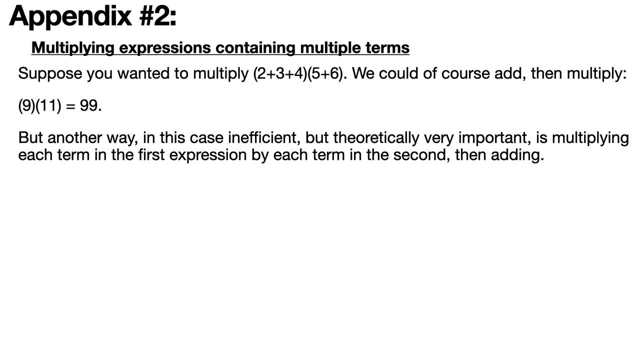 formula really is Appendix number two, multiplying expressions containing multiple terms. So this is about expanding algebraic expressions, and first we're going to do a concrete example. that might be kind of insultingly easy, but it's good to do things concretely first. 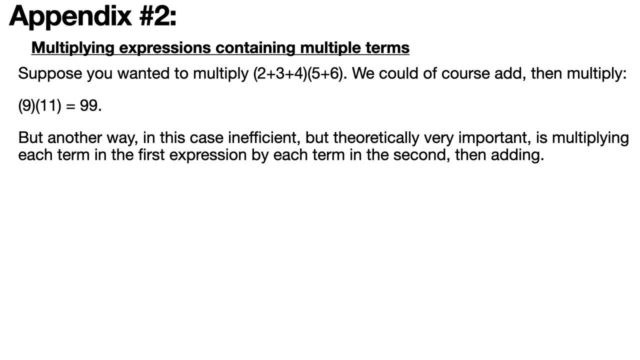 and then algebraically. So suppose you want to multiply 2 plus 3 plus 4, that whole thing times 5 plus 6.. And most people in circumstance would add first: 2 plus 3 plus 4 is 9, 5 plus 6. 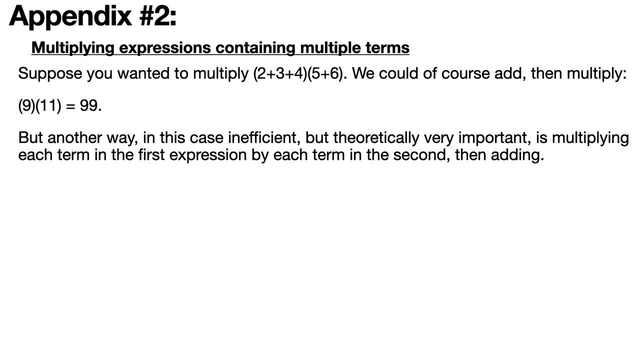 is 11, and you multiply to get 99. But the other way is important. The other way is: first you multiply every term in the first expression by every term in the second, and then you add all of them together And teachers teach this in different ways. I'm very partial to teaching. 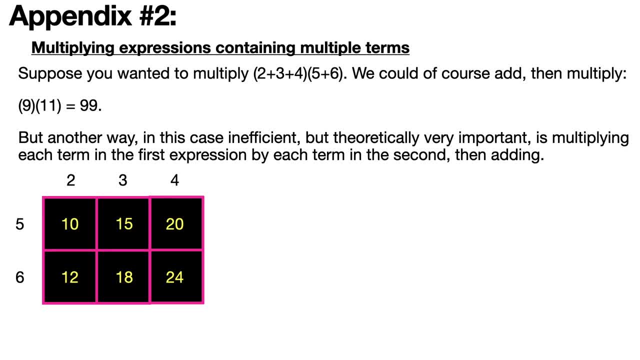 it with a box. Even though it's inefficient, it really gets the idea across. So when you multiply, you're really finding the area of something, And so you write all the terms of the first part on the top and all the terms of the second expression on the side and you multiply all of these as if. 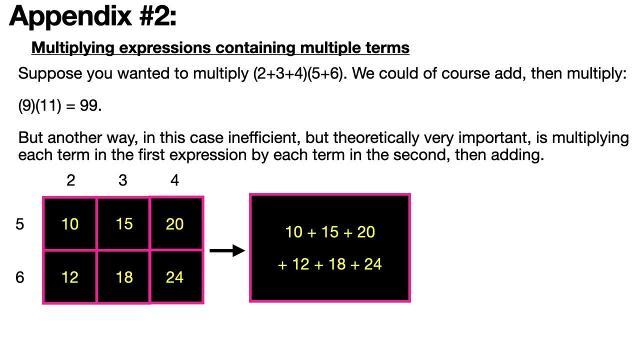 it was a little multiplication table. Then you'd add all the results and then you'd get 99, which is the same. Now, why would anyone do it this way? For numbers, it's really there's no point of doing it, except. 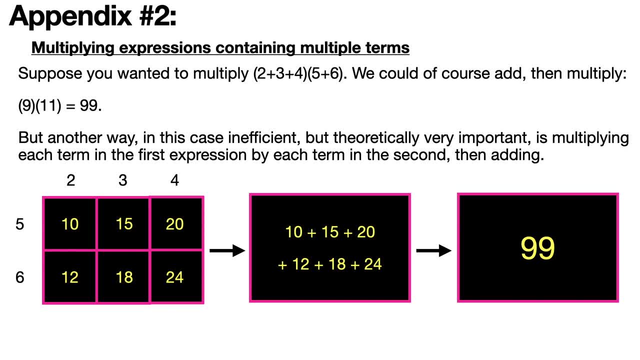 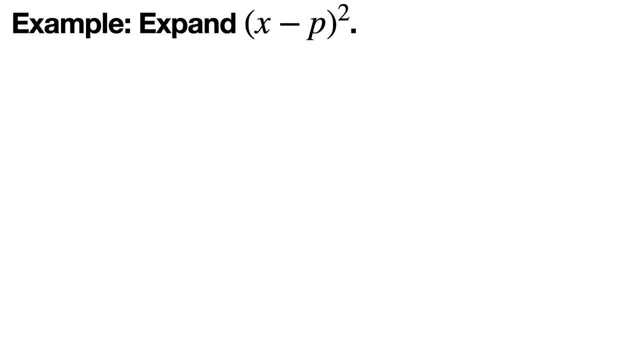